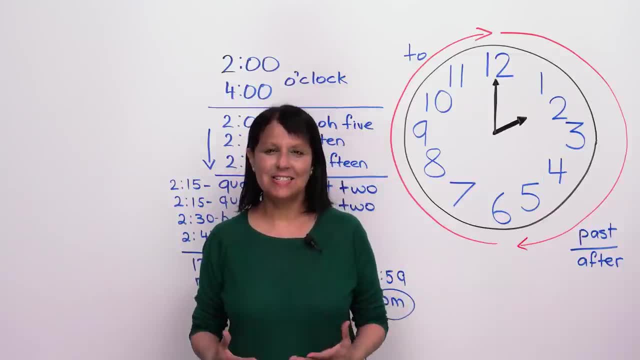 Hi, I'm Rebecca from wwwengvidcom. In this lesson we're going to learn how to tell time in English. Okay, So, for example, if someone tells you I'll meet you at 10 to 10.. What? 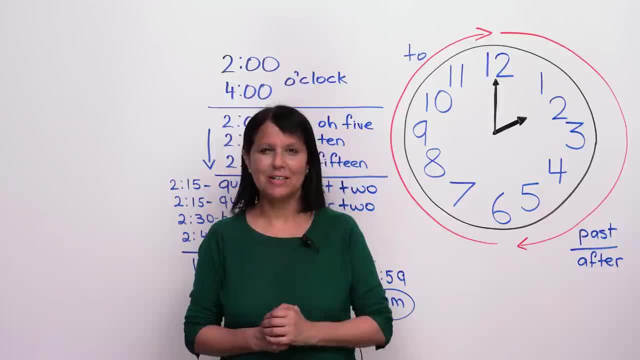 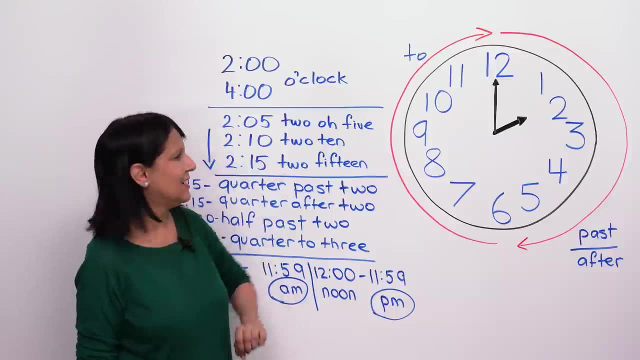 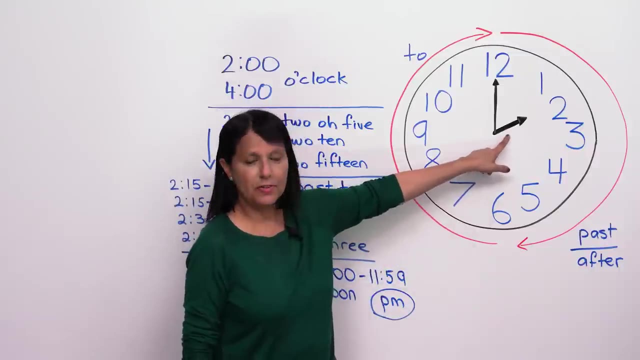 does that mean? What is 10 to 10?? We're going to find out. Okay, Let's go Alright. So here's the clock that I've drawn. Excuse my drawing, But what time does it say? Okay? So let's examine the clock. So this is called the hour hand. It shows the hour. 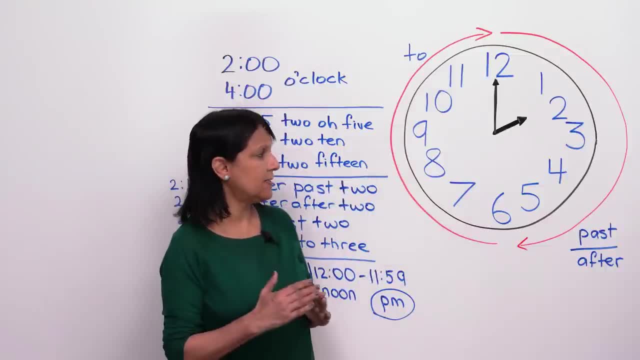 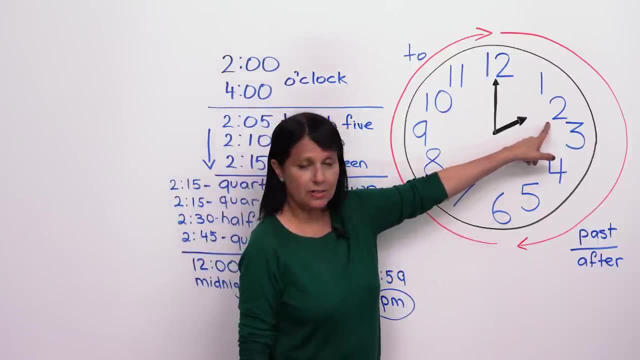 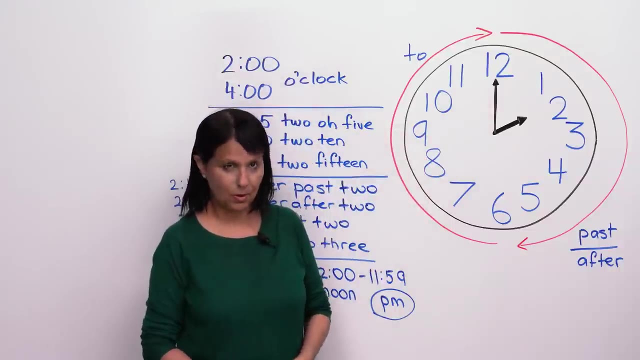 And this is called the minute hand. Okay, The shorter hand is the hour hand and the longer hand is the minute hand. Alright, And right now the hour hand is pointed to 2, and this is pointed to 12, so that means it is 2 o'clock, Alright, So, as we go around, it would be: 1 o'clock, 2 o'clock, 3 o'clock, 4 o'clock, 5 o'clock, 6 o'clock, 7 o'clock, 8 o'clock, 9 o'clock, 10 o'clock, 10 o'clock, 11 o'clock, 11 o'clock, 12 o'clock, 12 o'clock. 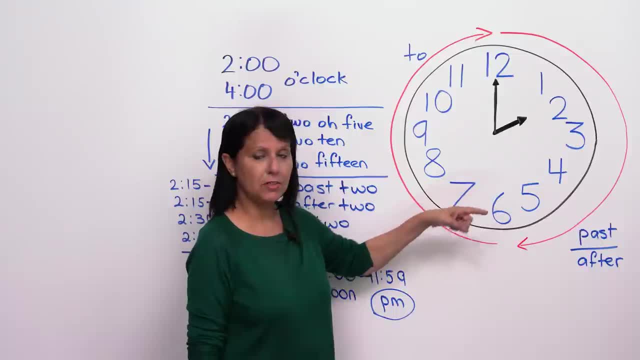 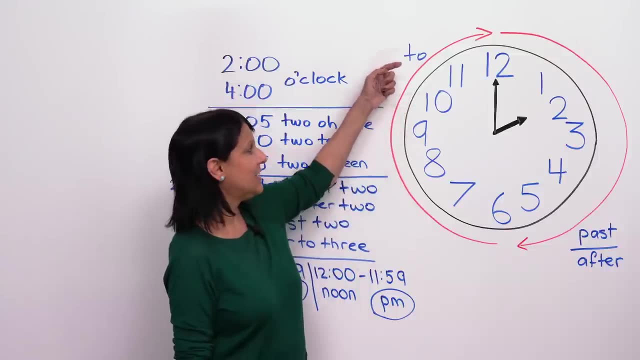 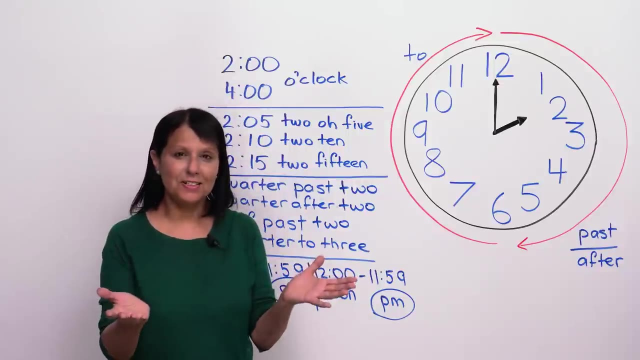 2 o'clock, 3 o'clock, 4 o'clock, 5 o'clock, 6 o'clock, 7 o'clock, 8 o'clock, 9 o'clock, 10 o'clock, 11 o'clock and 12 o'clock. Now, if you just say 12 o'clock, if you don't, 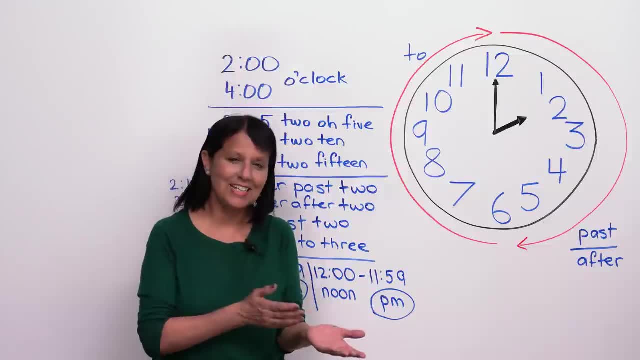 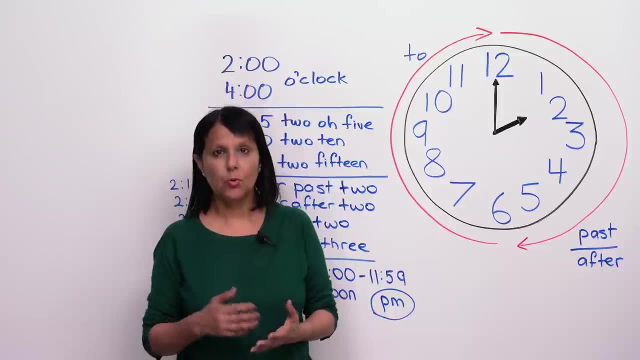 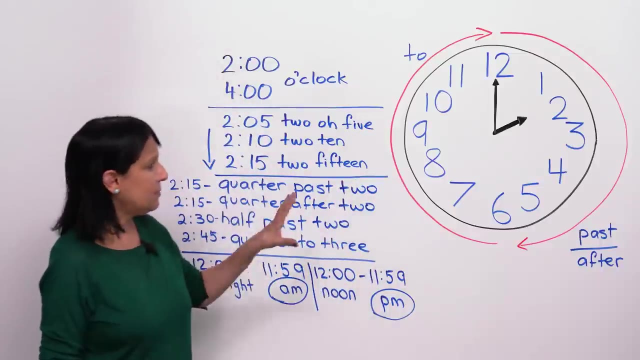 know what it's like outside. is it dark? Is it 12 o'clock at night? Is it 12 o'clock in the afternoon? So sometimes, when it's 12, we just say 12 noon Or midnight. Okay, If it's night we say midnight. But we'll get to that Now there. 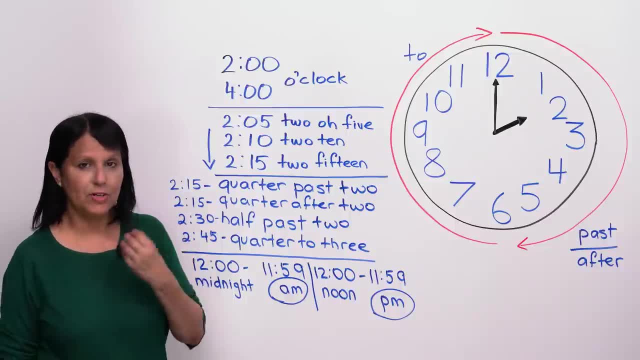 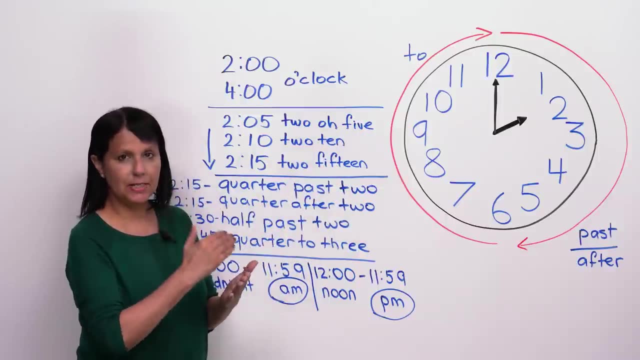 are many things you need to know in order to be able to say the time or express time correctly. Alright, So let's go through what they are. So, as I said, first of all, if it's a complete hour on the hour, then just say the hour, the number plus o'clock, Alright, 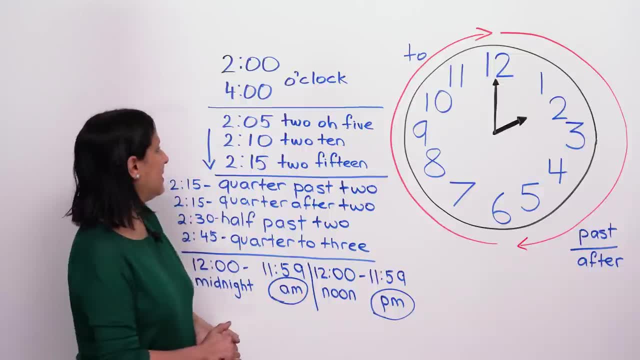 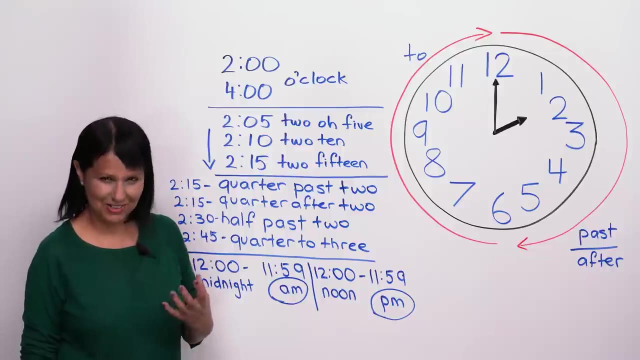 That's the expression: 2 o'clock, 3 o'clock, right, Then let's start going by 5-minute intervals around the clock and see what happens. So here we would say 2 o' 5.. Say it after me: 2 o' 5.. Good. 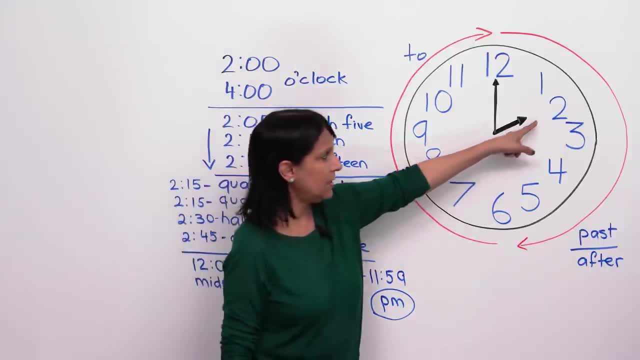 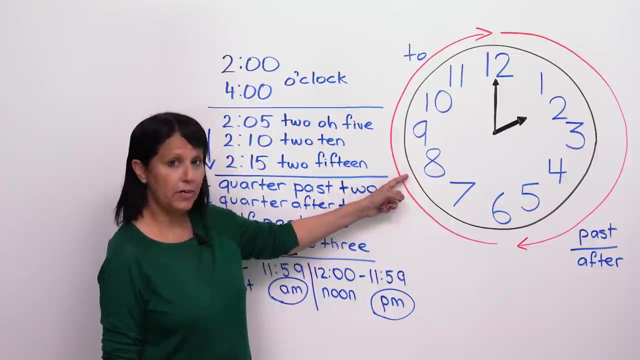 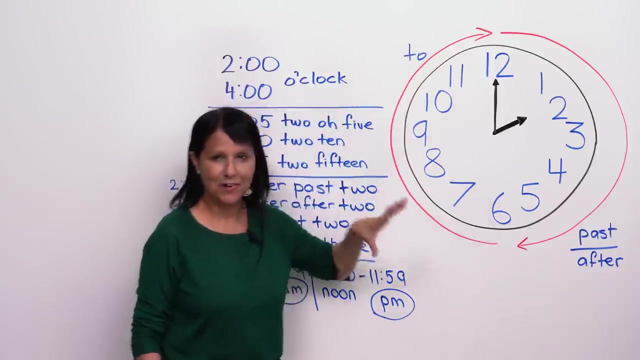 The next one: 2, 10.. Okay, That would be here, 2, 10.. Then here: 2 15,, 2 20,, 25,, 2 30,, 2 35,, 2 40,, 2 45,, 2 50,, 2 55. Okay, So we're going by 5-minute intervals right now, And it could. 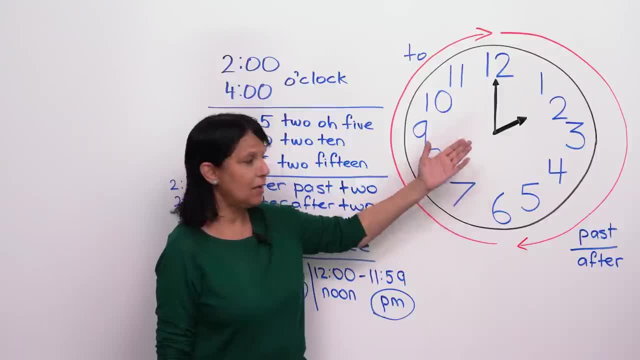 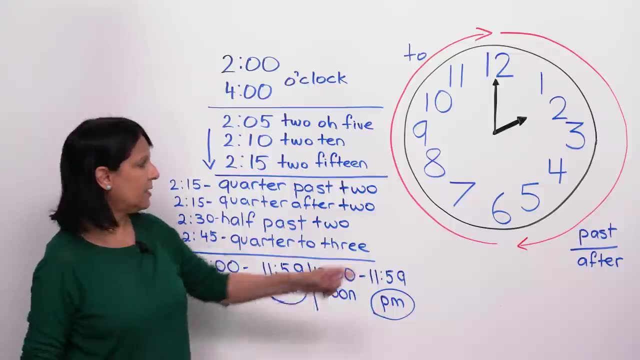 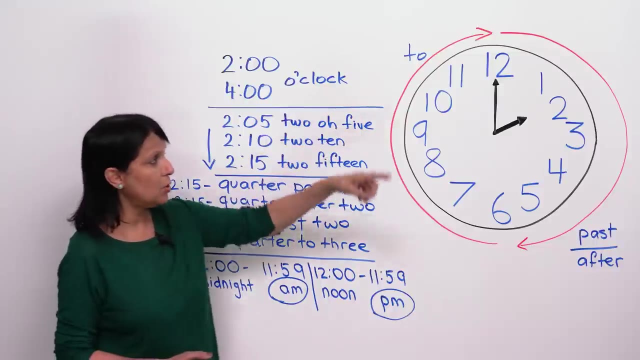 be something in between. It could be 2- 12,, or it could be 2- 23.. But usually people round off to those These numbers here. Okay, So one way that you can tell the time, and I think it's the easiest as long as you know. 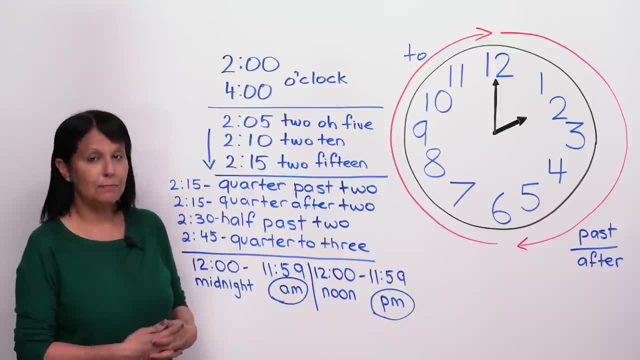 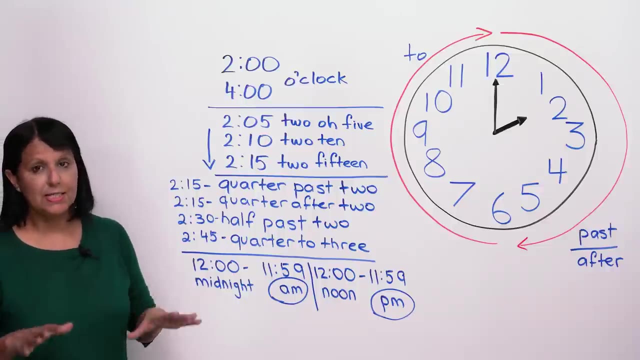 these basic numbers up to 59,, but certainly the numbers by 5, is just to say that 2 o' 5, what's the time? It's 2, 15.. It's 2, 50.. It's 2, 40.. Okay, 2, 45, and so on. That's the. 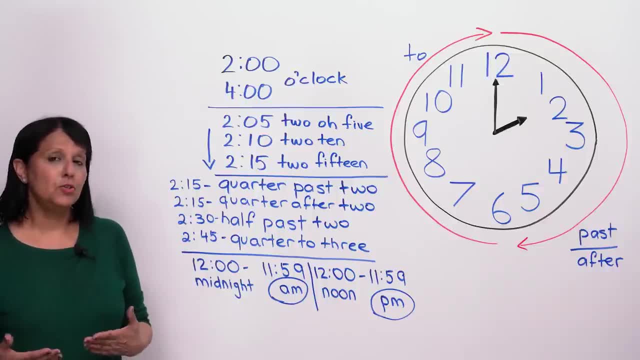 easy way And you can say that, but you might hear people using another expression or a few other expressions as well, So let me explain those to you. So, as I said, So what we're going to call 2, 15, or quarter past 2.. So why are we saying that? Because 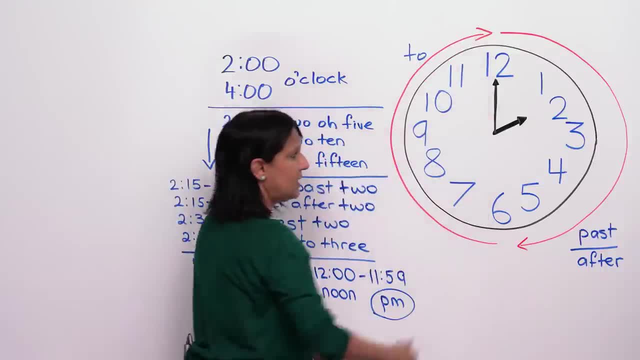 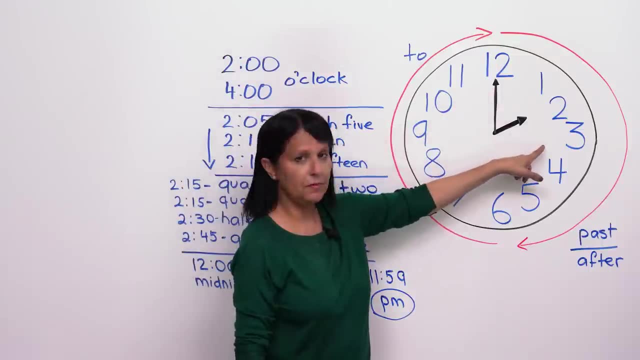 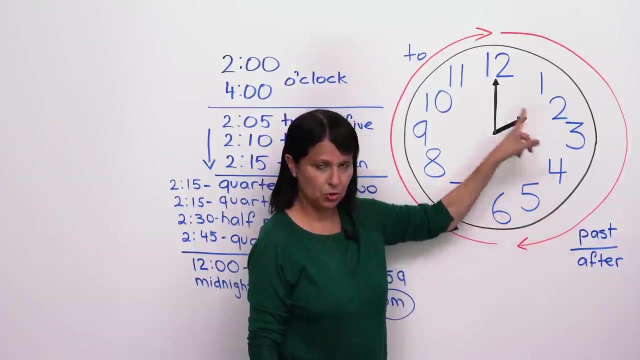 in this method, what we're doing is we're dividing the clock into quarters. Okay, Like this and like this. So when it's 2- 15,, it's a quarter past 2, or a quarter after 2.. After: 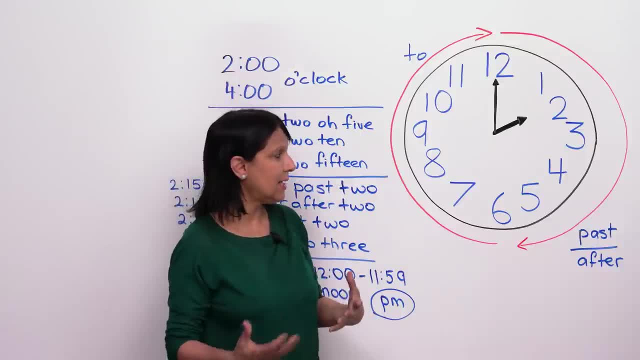 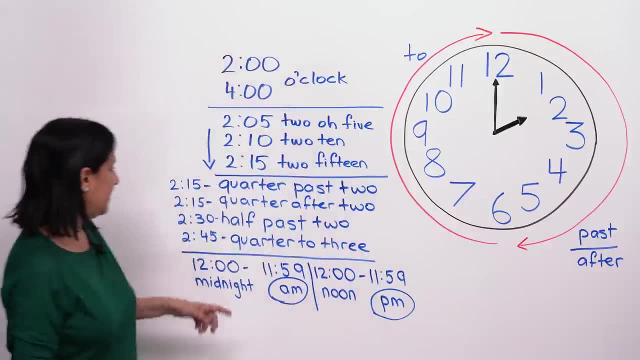 2 o'clock. So we don't have to say after 2 o'clock, We can just say at that point it's a quarter past 2.. It's a quarter after 2.. Okay, Then when it comes to 2- 30, we could say it's. 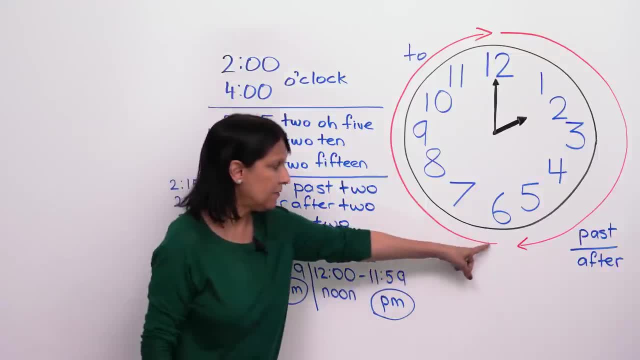 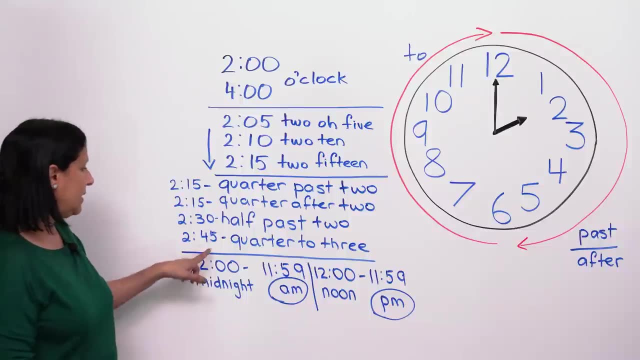 2- 30,. or we could say it's half, Right, Half, from the 12 to the 6. It's half past 2.. That's how we express that, And at 2- 45, we can also say it's a quarter to 3.. 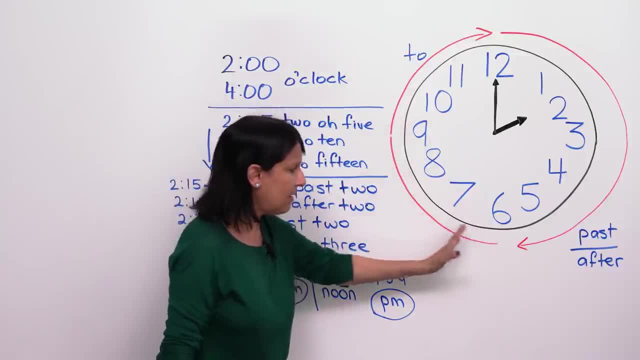 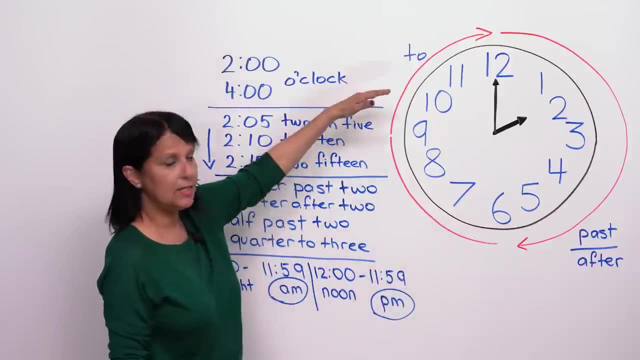 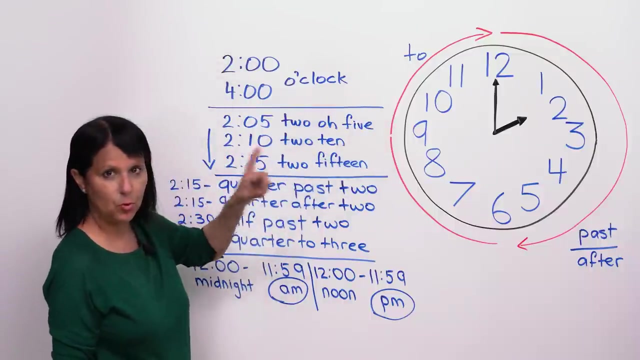 Quarter to Now, anything after the 6,. you see this other arrow here. From here to the 12, we have to say something to Quarter to 12.. Quarter to 3.. Okay, Would be quarter to 3 if it was 2, 45.. All right, Or 25 minutes to. 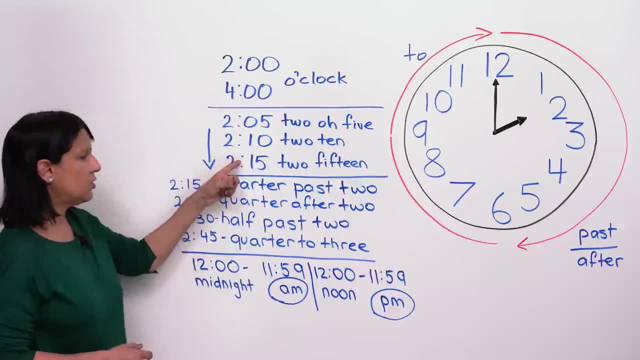 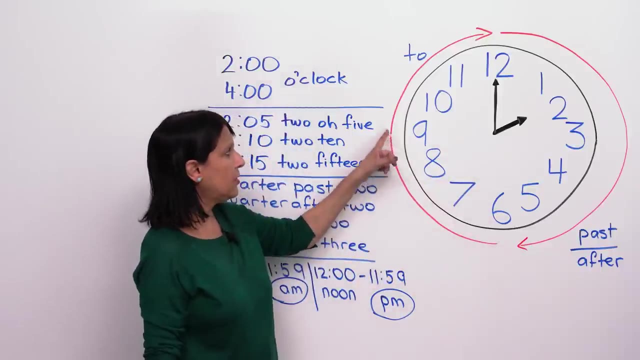 3.. You could say that, but those you'll probably just hear people saying 2, 35,, 2, 40, and so on. But on these quarter and half people do use these other expressions. Okay, So again, quarter past two, half past two, quarter to three. 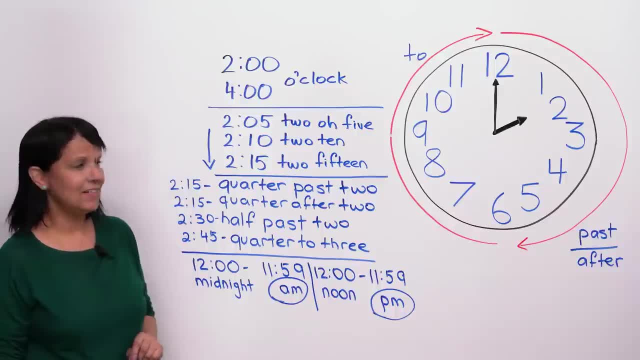 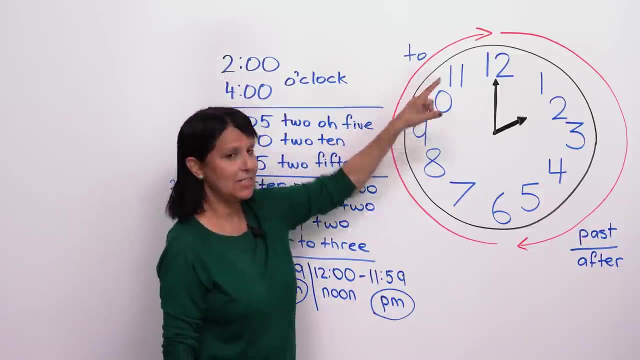 Okay, Now remember when I said ten to ten, So that was ten minutes to ten o'clock. Ten minutes to ten o'clock, All right, Ten minutes before ten o'clock. So when people say ten to ten, ten minutes to ten. 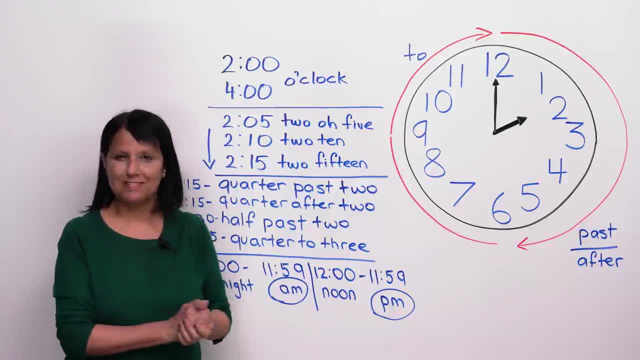 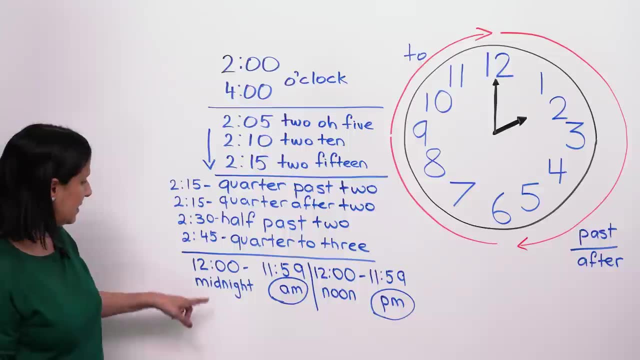 It's not used very often, but sometimes people just use it. in short, Okay, All right, Let's look at a couple of other things you might see when talking about the time. So when we're going from 12 midnight to about 11.59 in the afternoon, that period of time- 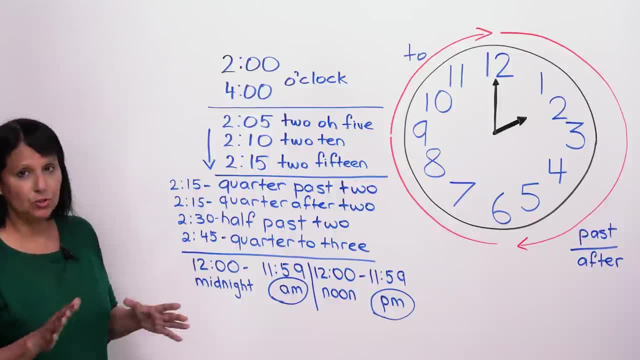 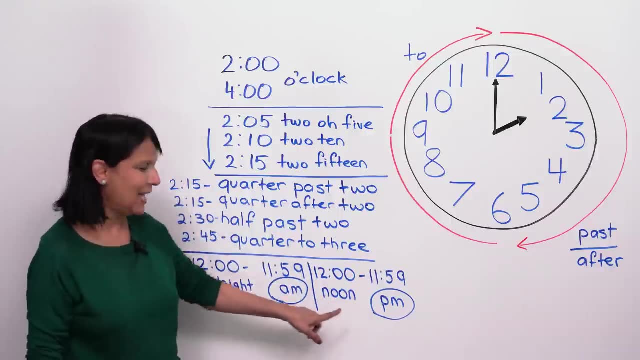 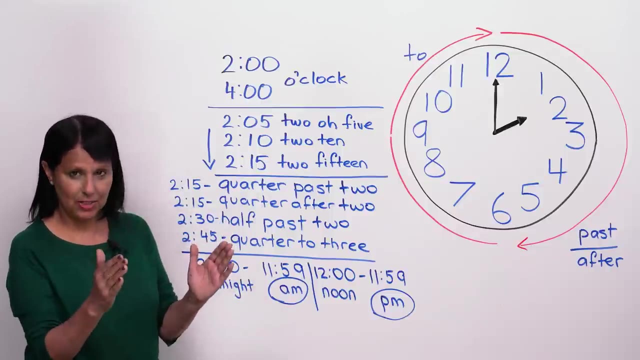 is referred to as AM- anti-meridiem, but don't worry about what it stands for. We'll just say AM and PM, Anti-meridiem and post-meridiem. Don't worry about those, Just say AM if it's from midnight to the afternoon and after 12 o'clock in the afternoon, 12. 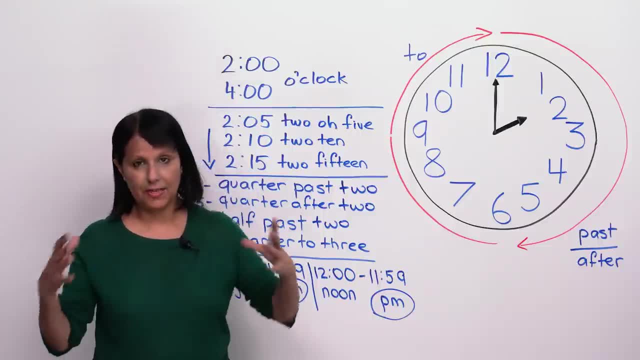 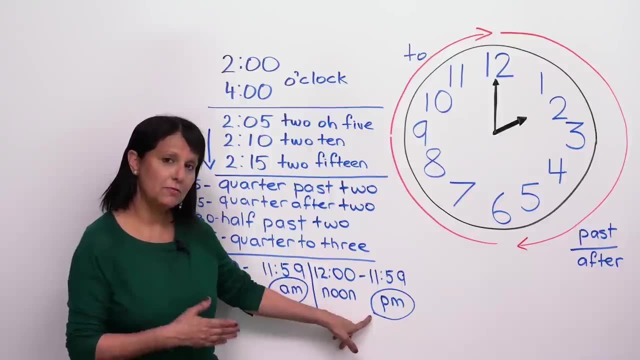 noon to 11.59 at night. we call that time PM. So if someone says I'll meet you at 4 PM, when is that? That's over here 4 o'clock in the afternoon. If someone says I'll meet you, 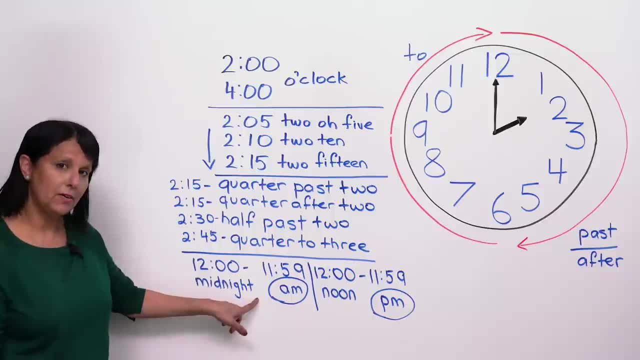 I'll meet you at 10 AM. that means over here right Ten o'clock in the morning. All right, I know it's a lot to take in. If you're a little bit unsure, you can study this for a while and then let's do a little. 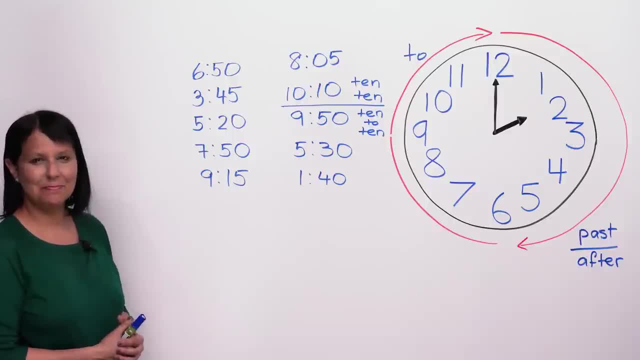 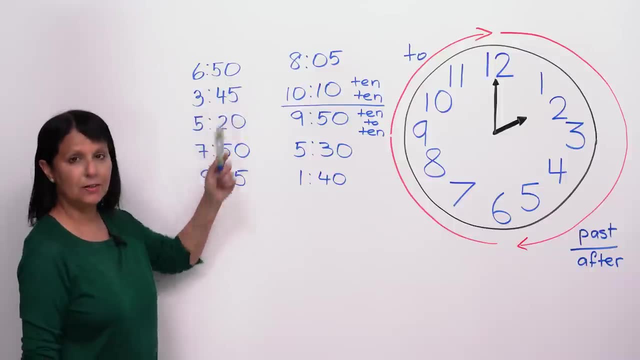 bit of a review, Okay, So are you ready to tell the time? Here we go, The first one. So what's the easy way we could say this: Six, fifty, Okay, Remember to say 50,, 50, short, not 15.. 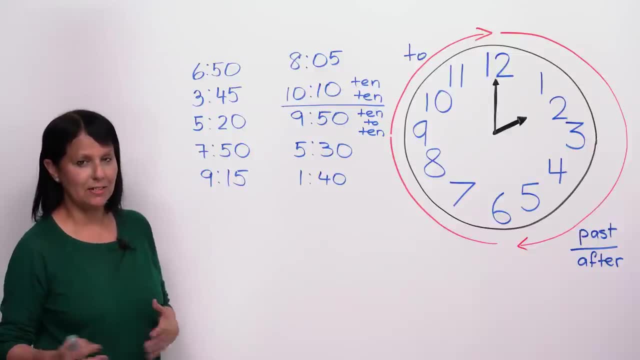 Okay, We're going to do something else, and somebody would get the wrong idea. Fifteen and fifty, Six, fifty or ten to seven. good, Three, forty-five or quarter to four, Five, twenty or twenty past five, twenty after five. 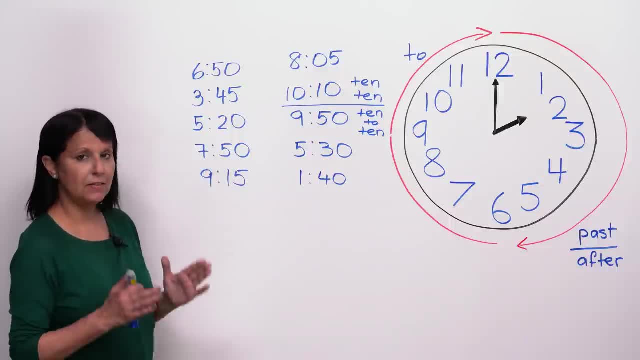 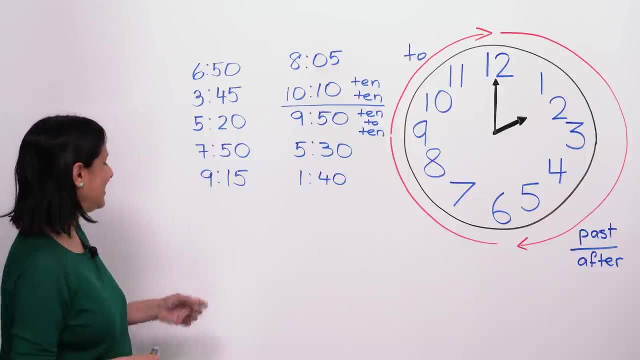 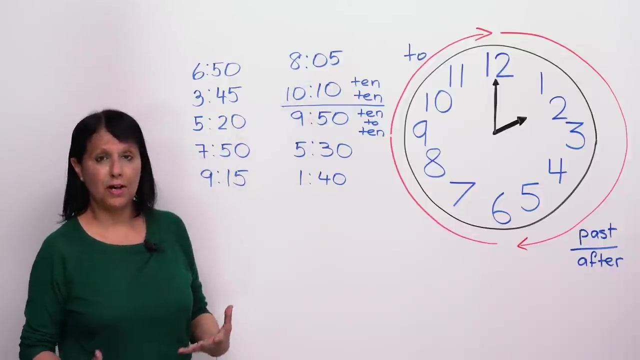 Seven, fifty, Okay, Nine, fifty, again fifty, or how would we say it? Ten to eight. good, Nine, fifteen, okay, now it's longer, nine, fifteen or quarter past nine, quarter after nine. Over here, eight o' five, usually we don't say, but you could say five past eight. 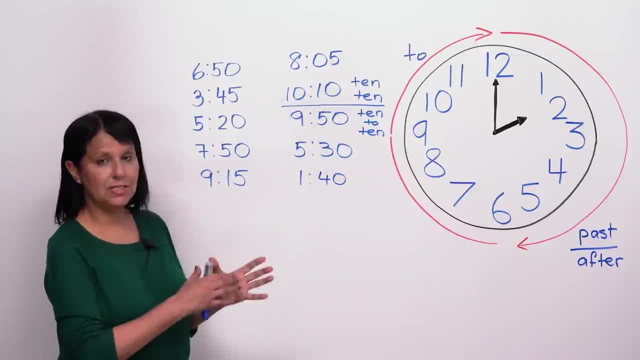 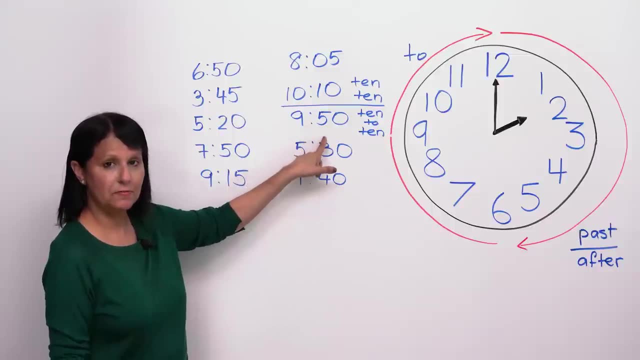 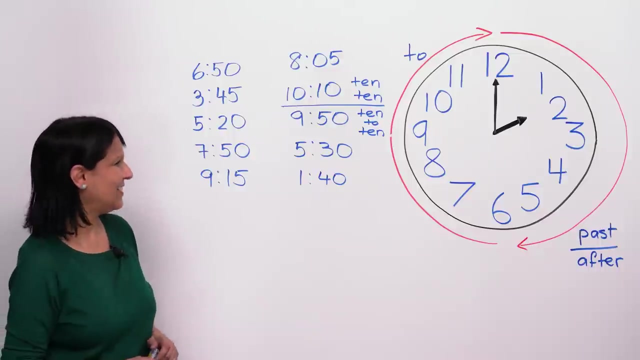 Now here, Half past ten. ten, which means ten minutes past ten o'clock. but this one, we would say either nine, fifty or ten to ten. ten to ten, Okay, Good, This one, five thirty, right. Or what's the other way to say that? 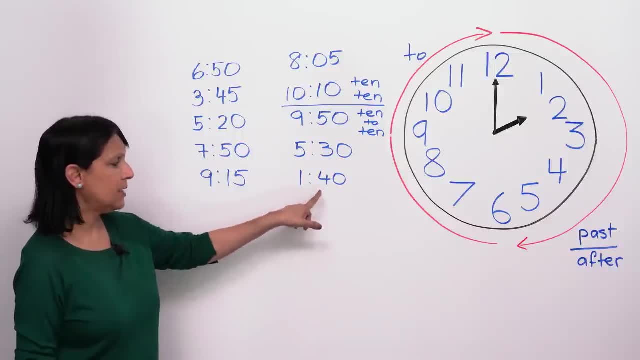 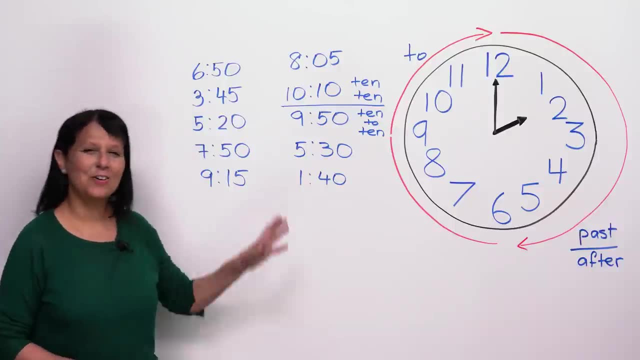 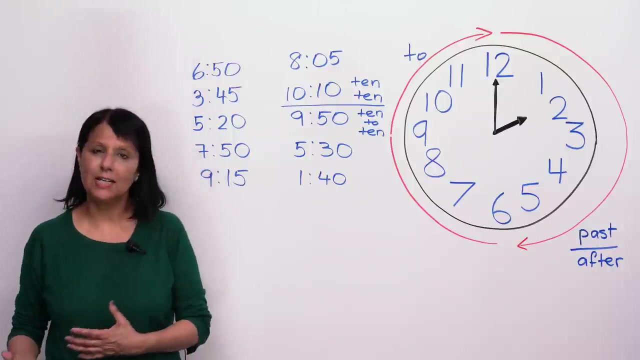 Half past five And one, forty or twenty minutes. Okay, Good, Twenty minutes to two o'clock, All right. So I know there are some variations, but learn to say the one which is easier for you, but learn to also understand all of the other options.